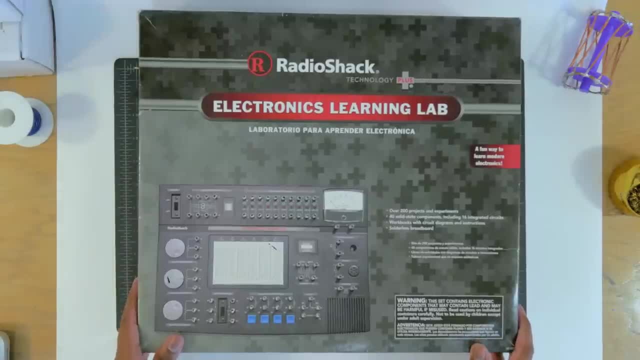 it all for me personally, And I've got like 5 or 6 different kits in my house. Now, before you exit out of this video and try and buy this kit for yourself, you can't. It's actually not available anymore. 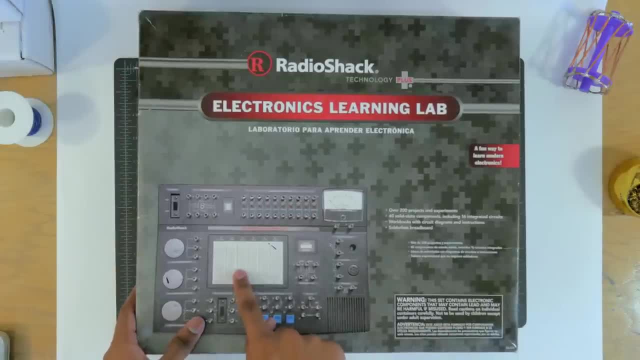 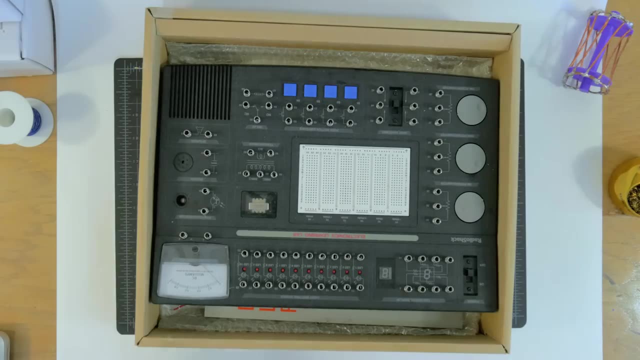 But don't worry, Stick to the end of the video and I'll let you know what you can do Now. why is a kit like this better, though, in the first place? Well, there's three major things, Three major takeaways that you want from every single good electronics kit. 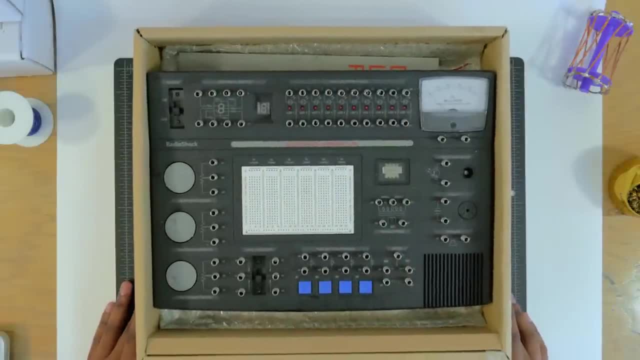 We can see the first one if we open this up and look right here. It's a breadboard. Now, learning how to use a breadboard is absolutely fundamental, And you can't get into electronics without knowing how to use a breadboard. 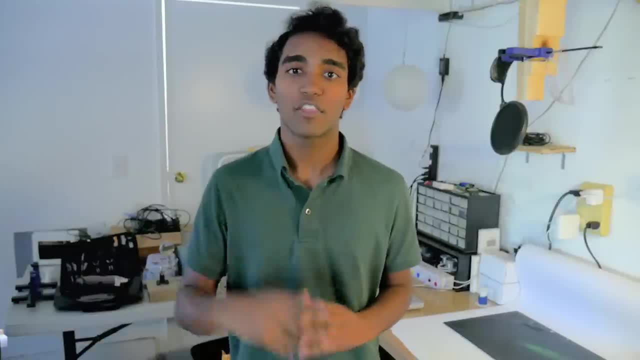 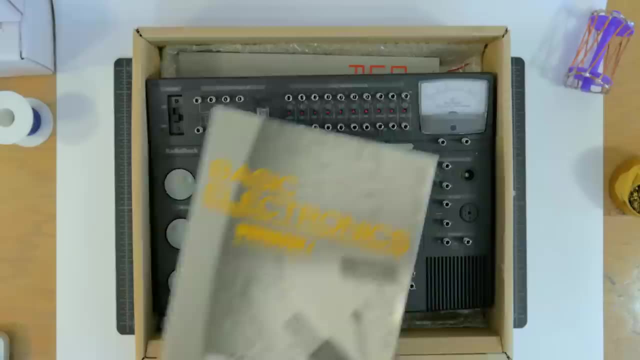 The reason for this is because any time you build a circuit in your life, the first 100 prototypes you do are going to be on a breadboard. I absolutely guarantee it. The other thing is that this booklet is very good. Now, it's far from perfect. There's a lot of things about it. 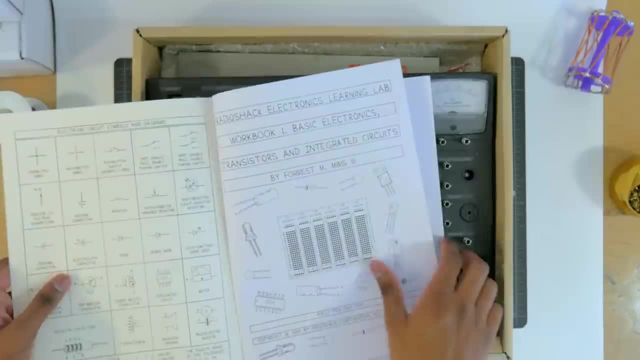 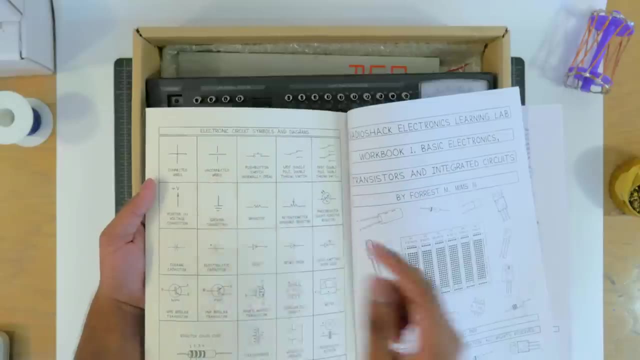 that I would change. But the one thing that it did really well is teach me how to read a schematic, And that is the second fundamental skill you need. If you can read a schematic, you can build any circuit you want. You can build a circuit. 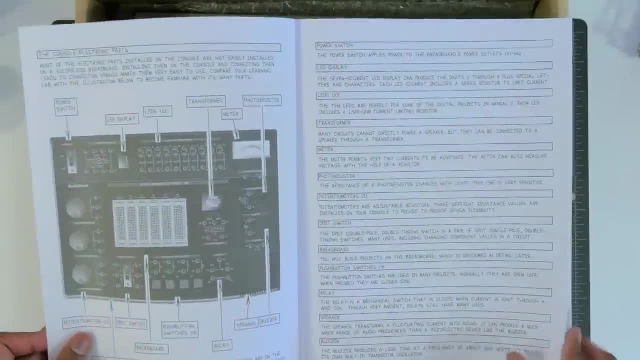 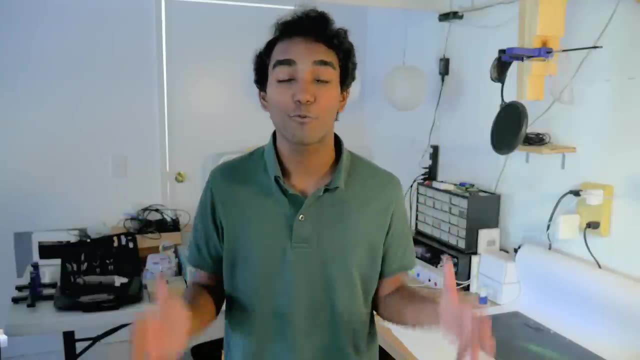 that does anything. Because you can go online, communicate with other electrical engineers online, see the circuits that they've made. because there's literally hundreds of thousands of different schematics for ridiculously cool projects all online And you can build any of them as long as you can read the schematic. 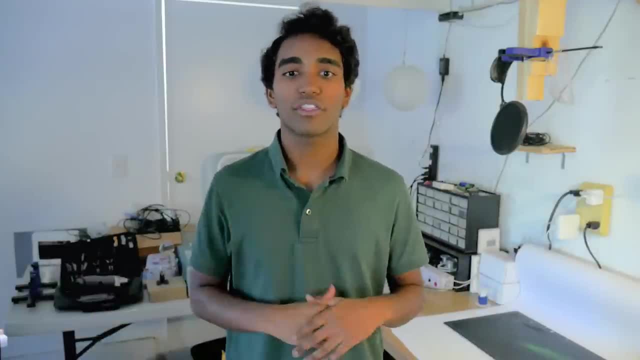 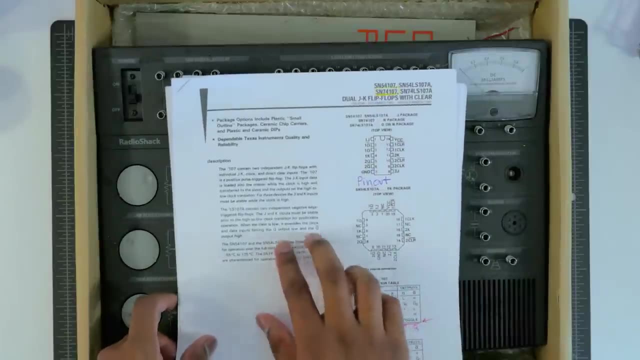 That's all you really need to know Now. the last really important thing is datasheets. Datasheets are amazing. Nothing is going to have more information than you thought you didn't need to know than a datasheet. Every IC transistor, BJT, has a datasheet, And if you don't know what it is, 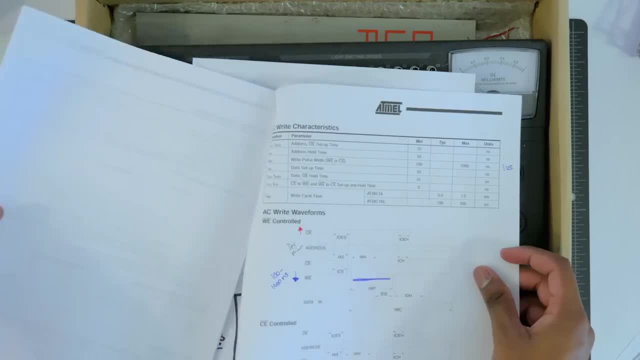 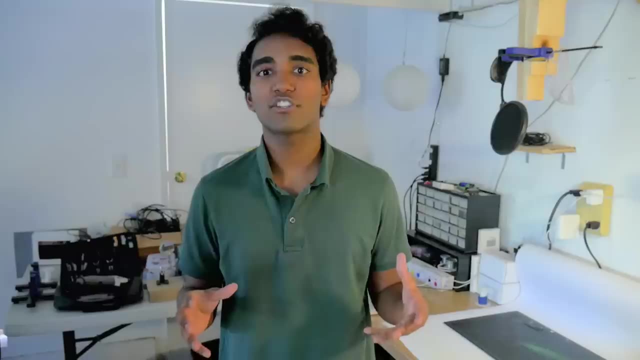 it's basically the manufacturer of a component releases this manual that gives all the properties and physical properties of this component. basically, Now, datasheets should have been mentioned in this kit's booklet, but it never was. The reason I learned about it, though, was because this kit, unlike so many, 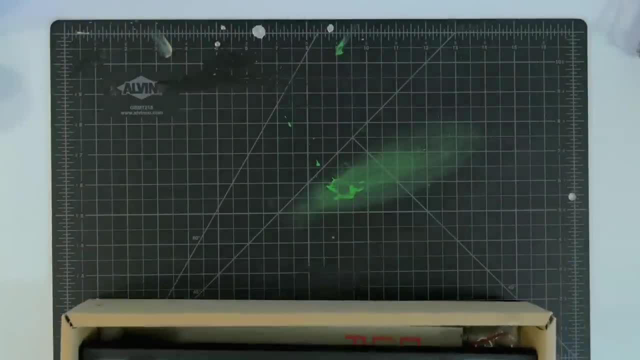 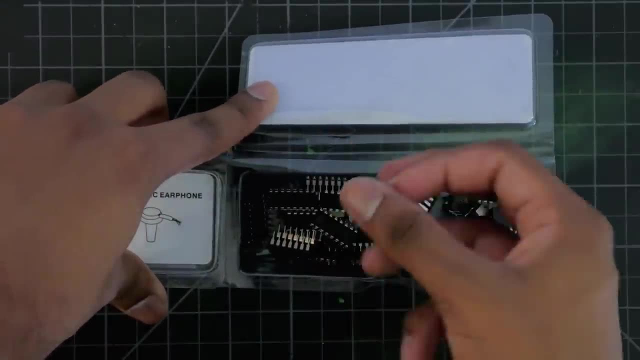 other kits that you find nowadays used real components, And that's huge, Because we weren't using Arduinos or Snap circuits with premade modules. We were using ICs, capacitors, resistors, components that real, professional electrical engineers would use. 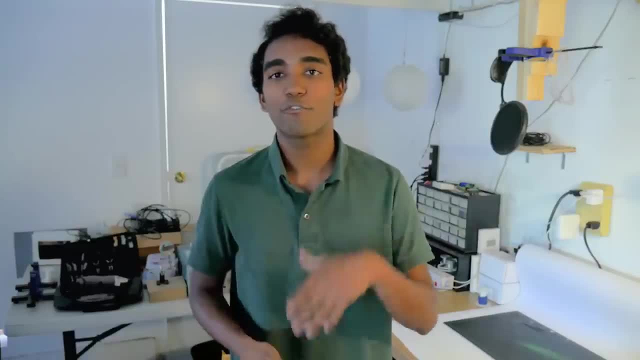 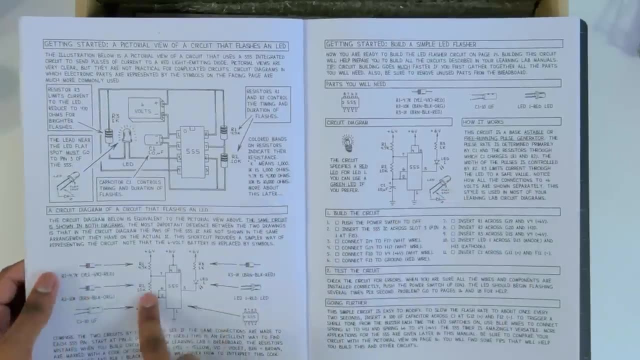 And in the beginning, yeah, it's super daunting. You don't know what you're doing. You know, if we open this book up and go to the first circuit, we can see the first real circuit I ever made. It's a 555 timer circuit. Now, I didn't know. 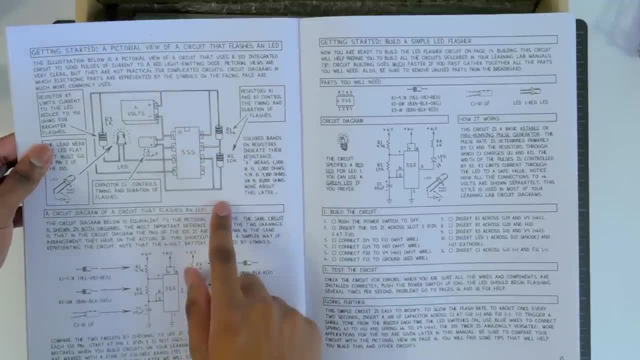 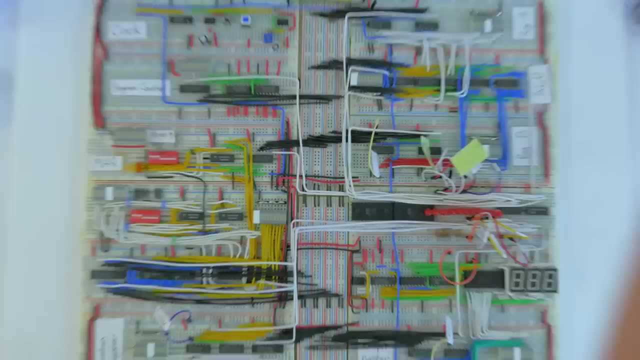 when I first built this circuit, how important it was or how ubiquitous it appears in electronics. But look at where we are now, Ten years later. we're doing our 8-bit CPU and the first thing we have to do is a clock module. 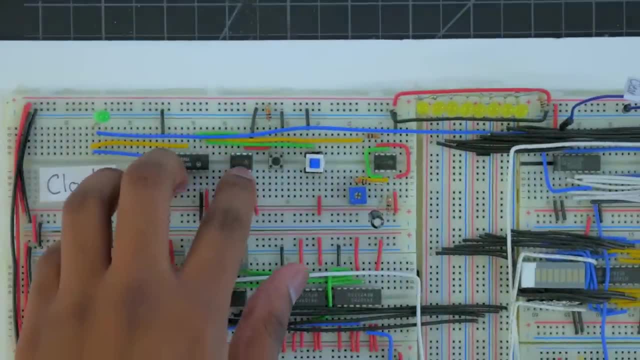 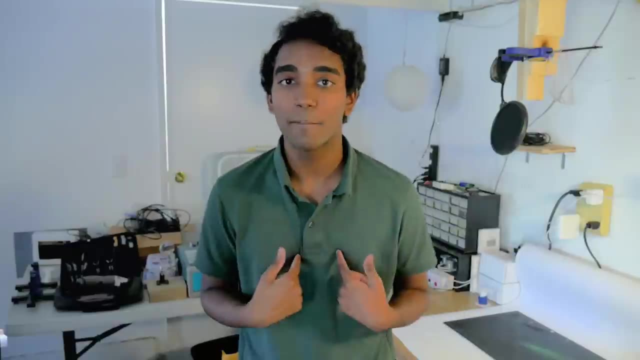 And that's based off a 555 timer. Then look at our next project, the decimal clock. The first thing we've got to do for that is start off with a 555 timer. This circuit is incredibly important. My first time building it, I didn't even know what I was doing. 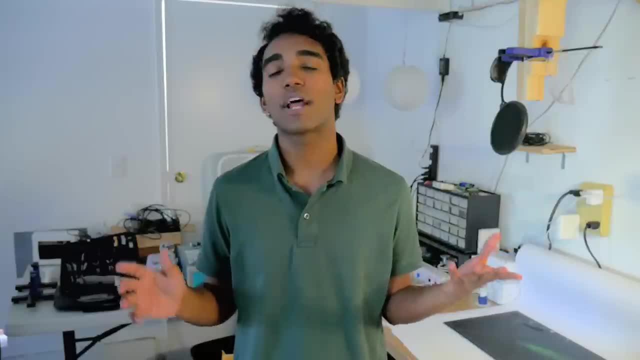 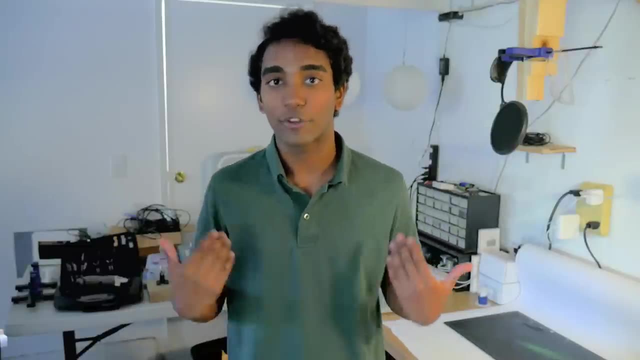 I had to put it together and take it apart probably 20 times And I didn't even know what I was doing differently each of those 20 times that I tried to put it back together, But eventually it worked one time, And now we're here. 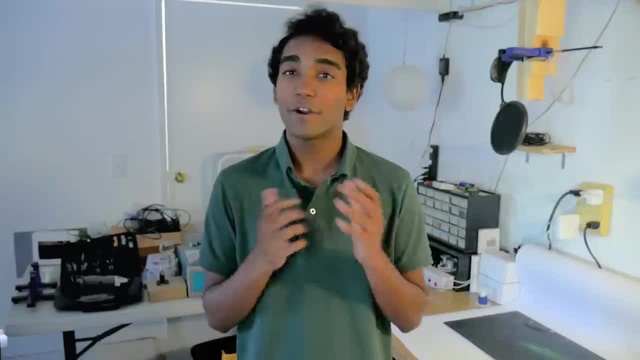 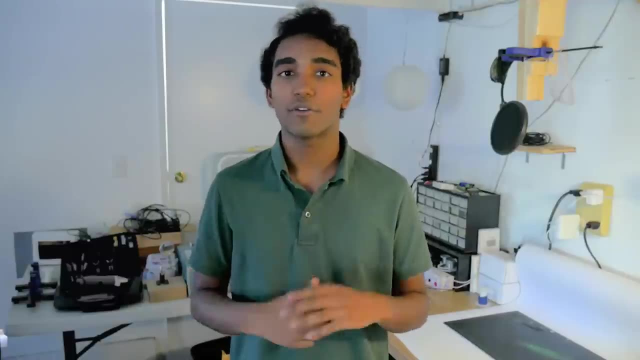 Now if you want to get into electronics, you're kind of out of luck. They don't make this Radio Shack anymore. Radio Shack went out of business a long time ago And if we look up on Amazon like beginner electronic kits or basic 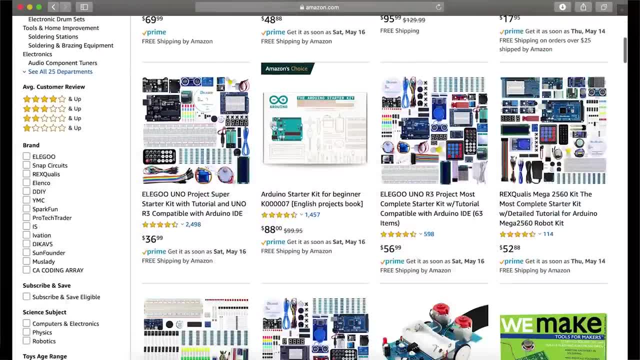 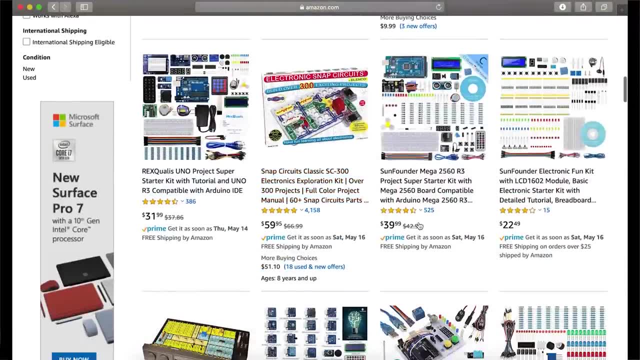 electronic kits, you can see that there really isn't that much available. We have these sort of snap circuit kits that aren't going to teach you much, And then we have these Arduino kits, which I really don't recommend for beginners. The problem with trying to learn basic electronics with an Arduino is that you're transforming. 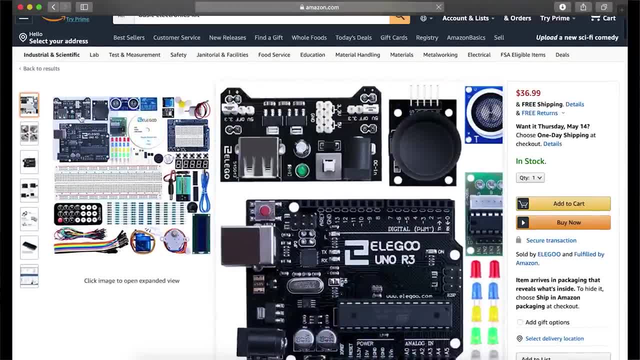 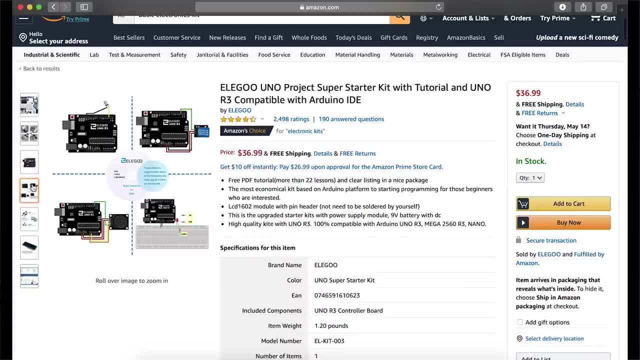 every single hardware problem you're trying to solve into a software one. So now you're not going to be learning about schematics or data sheets, ICs or transistors or anything like that with an Arduino kit. Now, a lot of these Arduino. 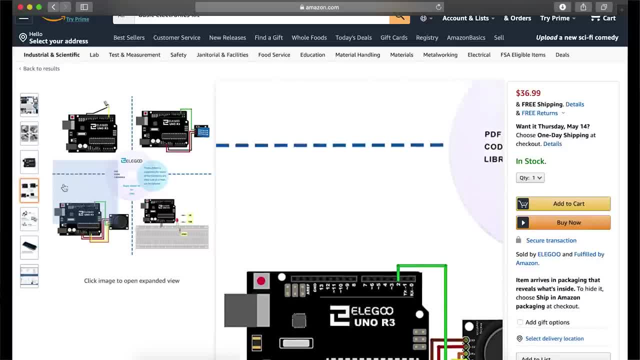 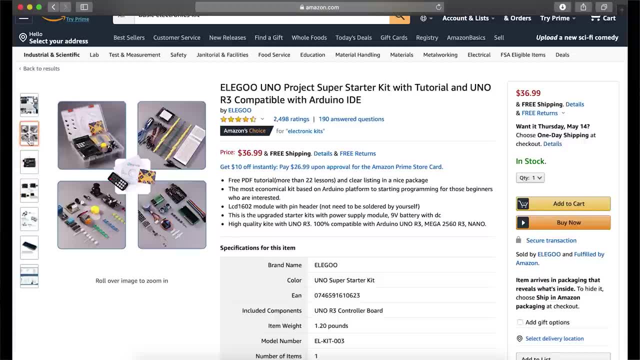 kits market really great because there's a lot of projects you can do with them. And that's just because Arduino is a microcontroller just like a computer, And just like a computer. there's a lot of things you can do with them, But you're not going to learn a lot about electronics. 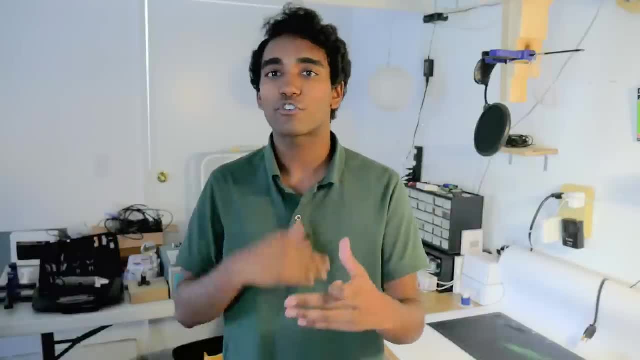 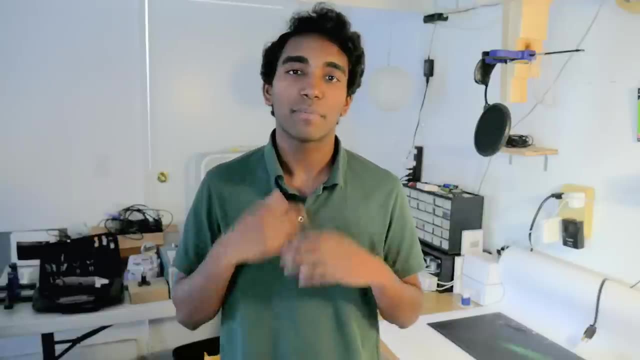 specifically, necessarily, You might use a breadboard a bit, but you're not going to know enough to be able to keep up with a lot of the YouTube videos you see online, or even some of the videos you see on this channel. Because of this, I was thinking that 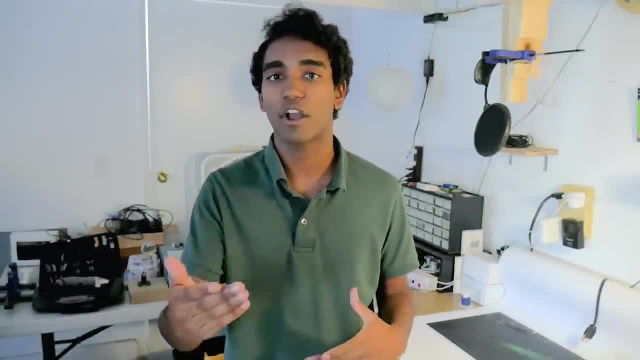 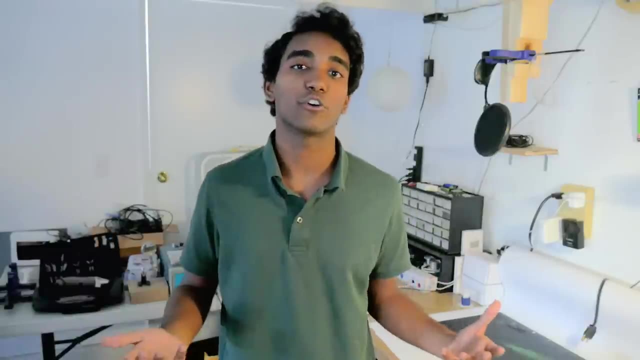 I might make my own beginner electronic kit for some of my subscribers, Just because a lot of my subscribers have been asking me for something like this And, honestly, I think that a kit is one of the best ways to learn beginner electronics. And when I go online and look at